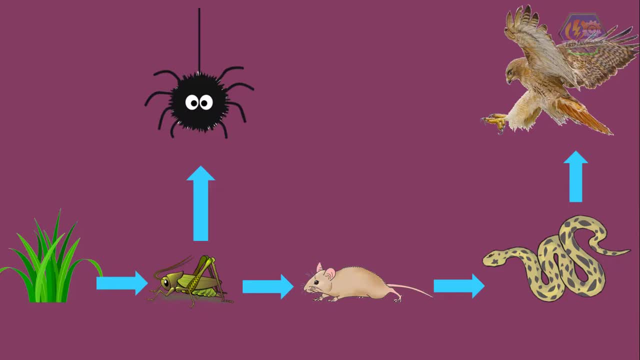 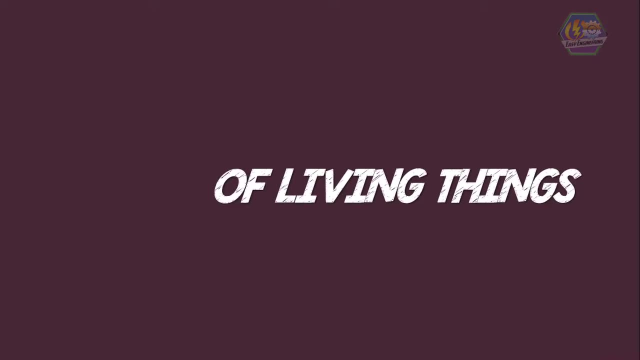 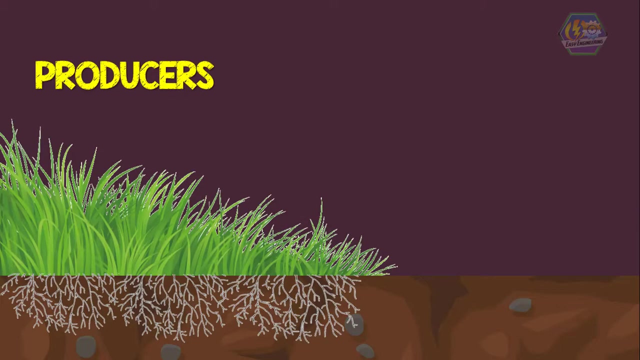 Like this spider. Then that forms another chain. Now there are different types of living things. There are different types of living things depending on how they use energy. First are the producers. Plants are producers because they produce energy for the ecosystem. They use water, nutrients from the soil and water. 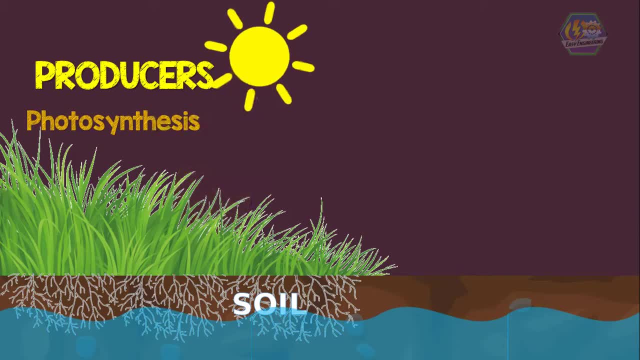 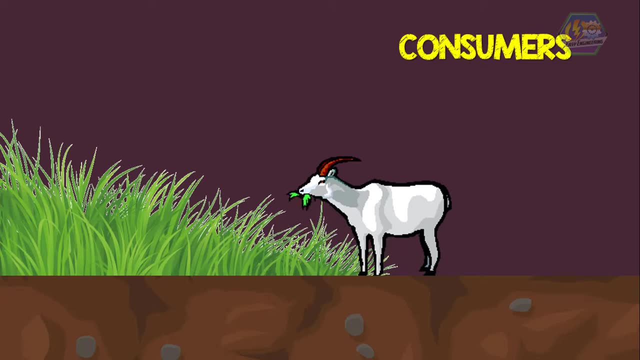 Then they absorb energy from sunlight through photosynthesis. Next are the consumers. Animals are consumers since they don't make their food like the plants. Instead, they eat the plants, And some animals eat other animals. Animals that eat fruits, vegetables or just plants are called herbivores. 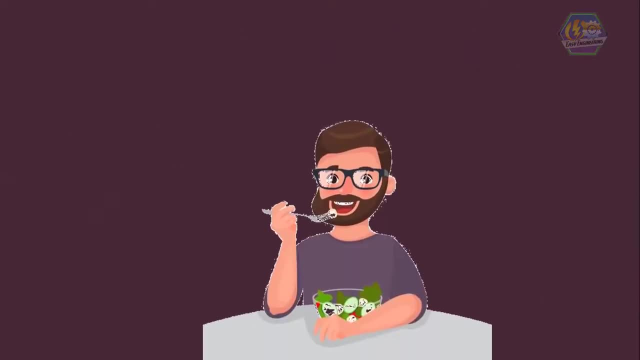 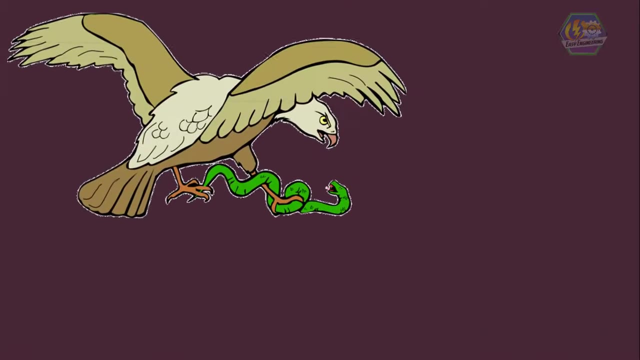 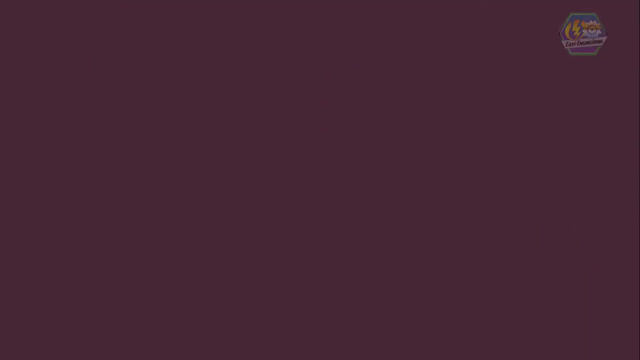 They are also called primary consumers. You can be one too, if you choose to be a vegan. Animals that eat meat only of other animals are called secondary consumers or carnivores. Now, if another animal eats another carnivore, then it is called a tertiary consumer. 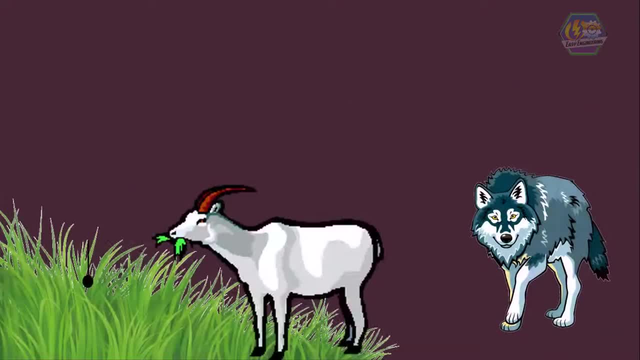 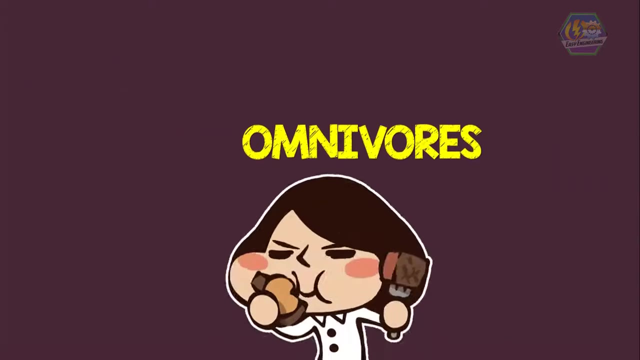 In the previous example, the grass is the producer, the goat is the primary consumer and then the wolf is the secondary consumer. Some animals eat both plants and animals. They are called omnivores. We humans are also omnivores, since we apparently eat everything. 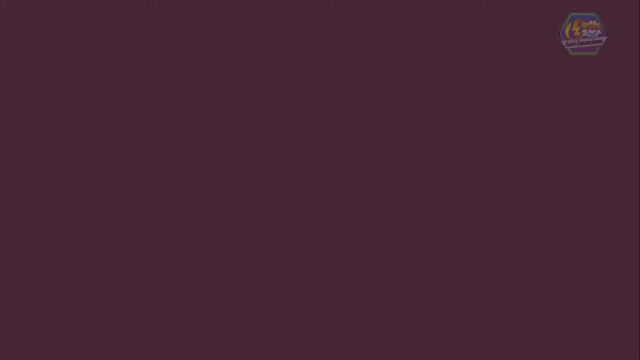 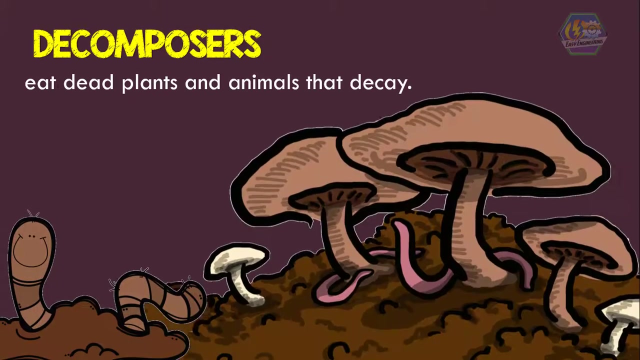 Lastly, the decomposers. They eat dead plants and animals that decay. They help put nutrients back into the soil for plants to eat. Some decomposers are the worms and fungi. Plants eat decomposers' nutrients. Then animals eat plants. 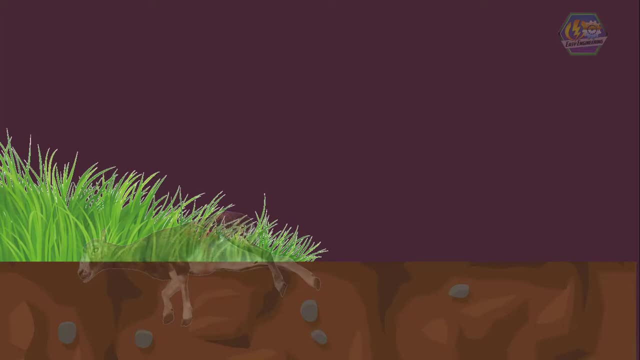 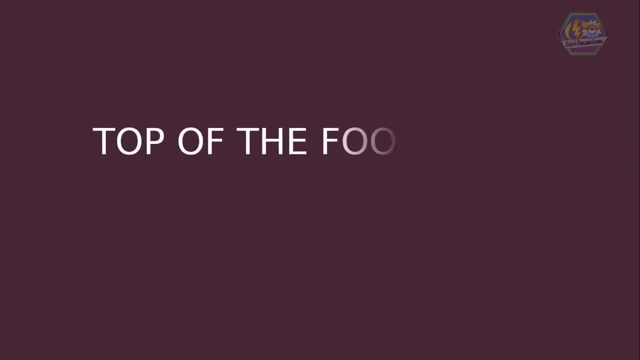 And if the animals die, they decompose. This cycle repeats over and over. Fun fact learners. did you know what's at the top of the food chain? Those are animals that no one eats, since they are either big or very strong to go up against. 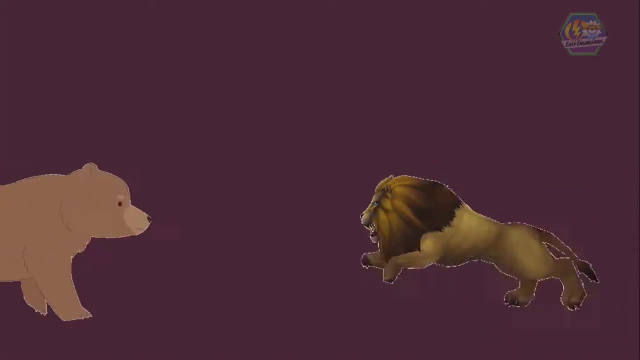 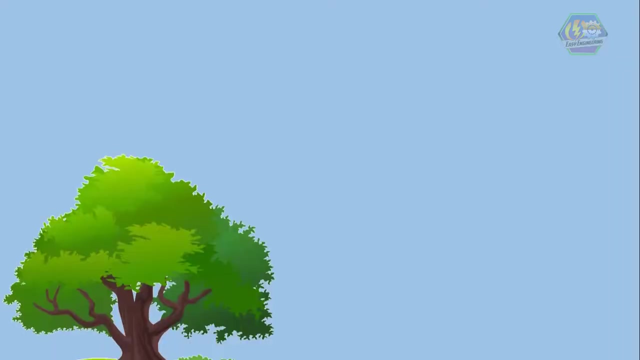 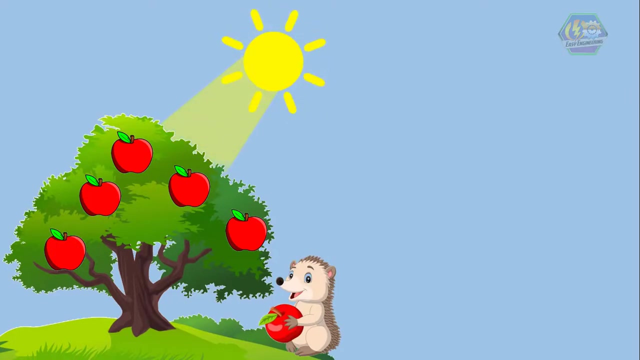 These are the lions, bears and orcas. They are the kings of their own jungle. Well, plants convert energy from the sun to a form of food, But every animal uses food as a source of their energy for their day-to-day activities. 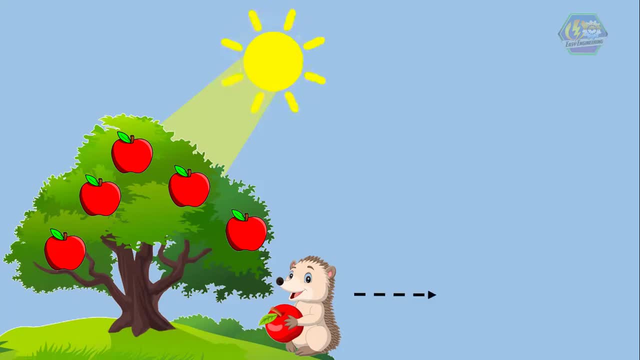 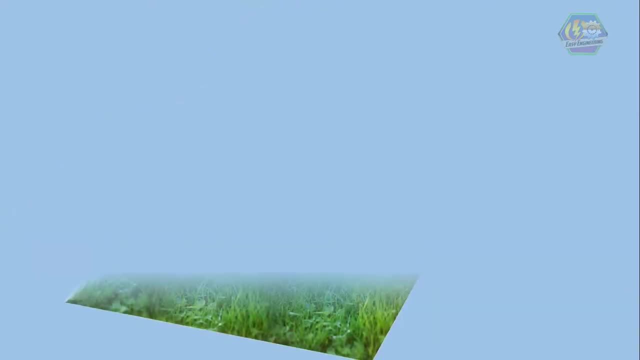 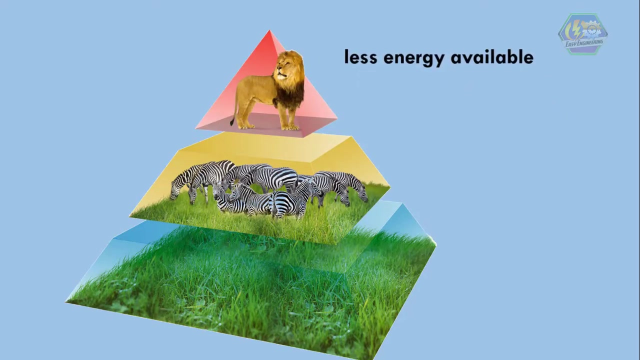 So if an herbivore gets eaten by a carnivore, the carnivore gets less energy, Just like the rest of the food chain. So as you move to the top of the food chain, there is less and less energy available. That's why there's only very few kinds of animals at the top of the food chain. 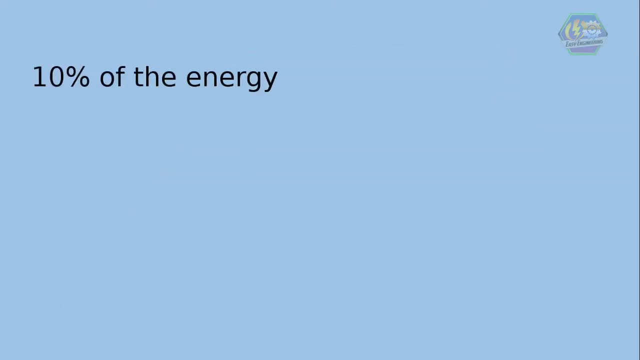 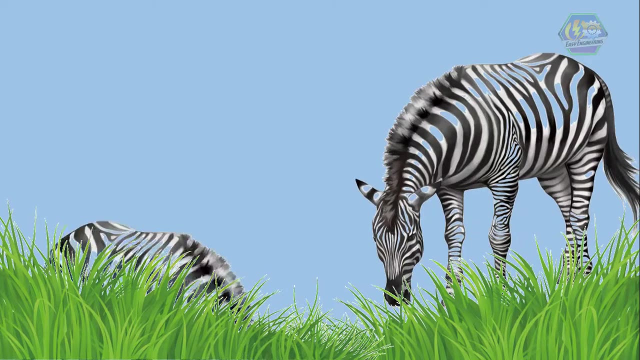 In fact, you only get 10% of the energy provided by plants if you eat animals. Like. there are a lot of grass available, then there's also a handful of zebras, But the lions are quite, very less than the number of zebras. 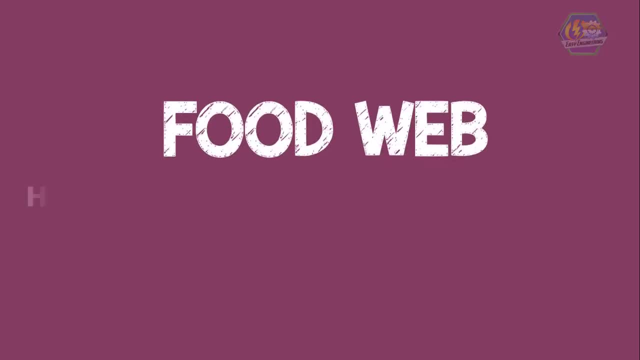 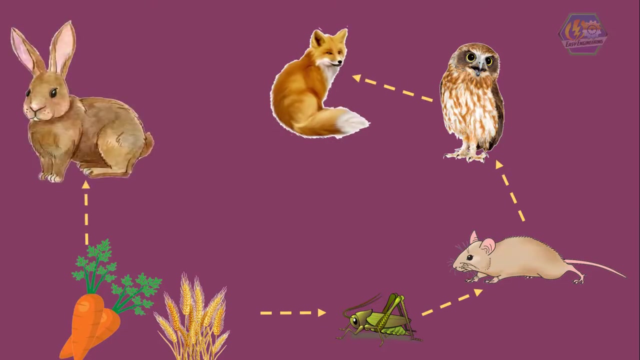 So how about the food web? How does it differ from the food chain? As we said earlier, there are many food chains in the environment. Any plant and animals can be part of another or several food chains. When you draw all the chains together, they form like a web called the food web. 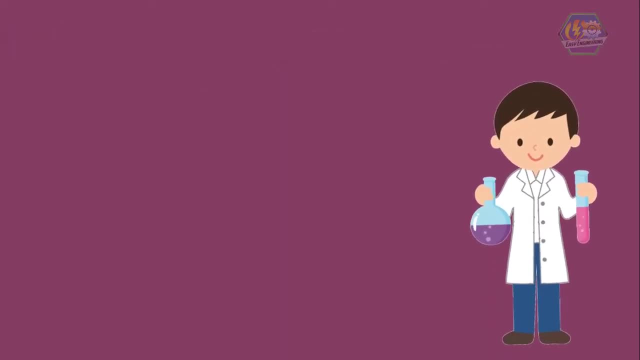 Scientists describe each level of food chain as the food chain. There are three levels in a food web with a trophic level. It might be very familiar, since it's almost the same in the food chain. In level 1, there's the plants or producers. 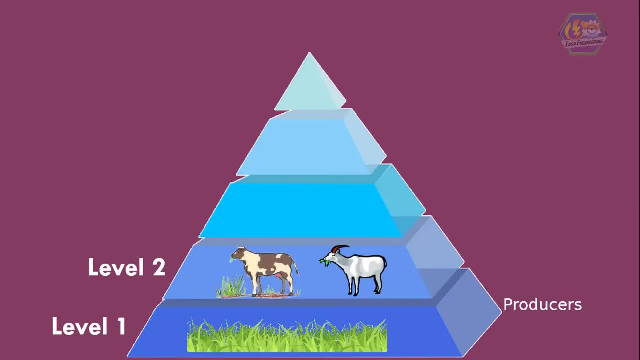 Level 2 are the animals that eat plants, the herbivores or primary consumers. Next is the level 3, or the animals that eat herbivores or secondary consumers, which are carnivores. Animals that eat carnivores or the tertiary consumers are carnivores. 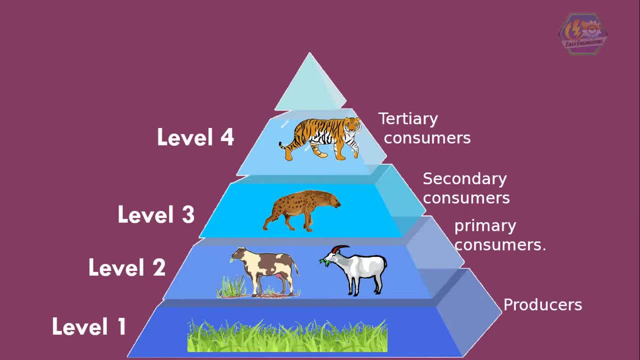 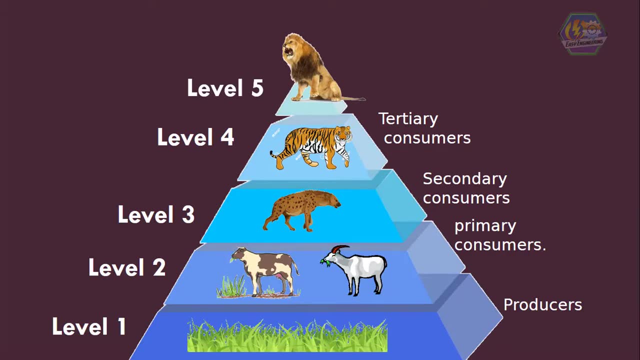 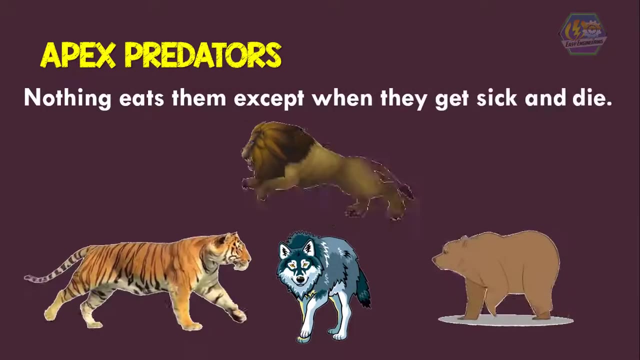 And still. carnivores are in the fourth level, And there's level 5, the animals at the top of the food chain. These animals are also called apex predators. Nothing eats them, except when they get sick and die. If we are strong enough, we could be apex predators too.